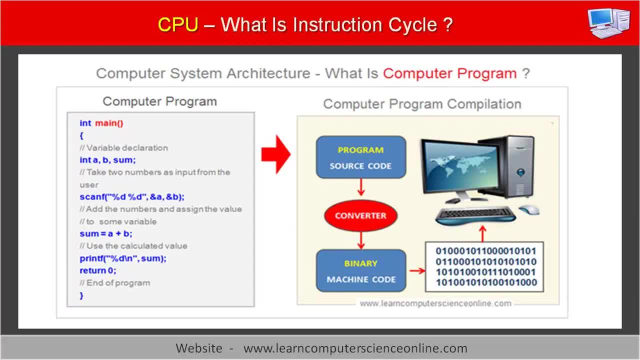 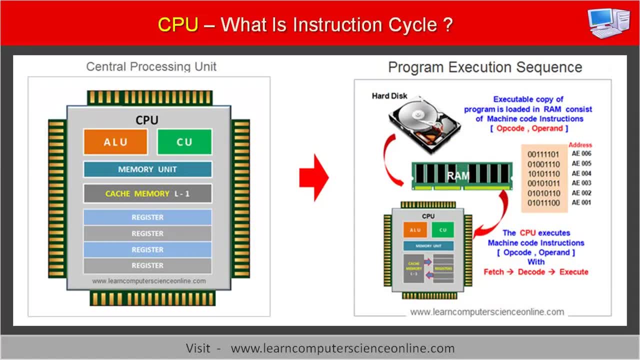 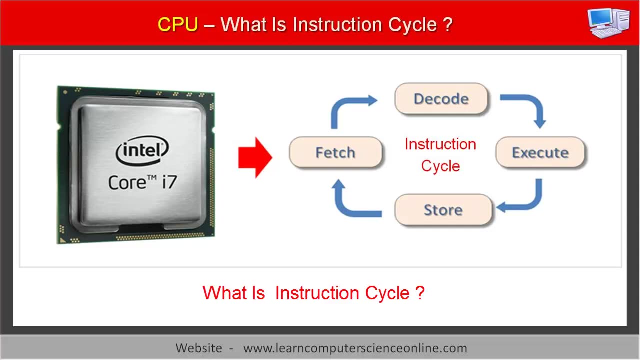 The computer program consist of set of machine instructions. The central processing unit, CPU, is responsible to execute These program instructions. In this tutorial you will learn what is instruction cycle and how it is related to the machine cycle. 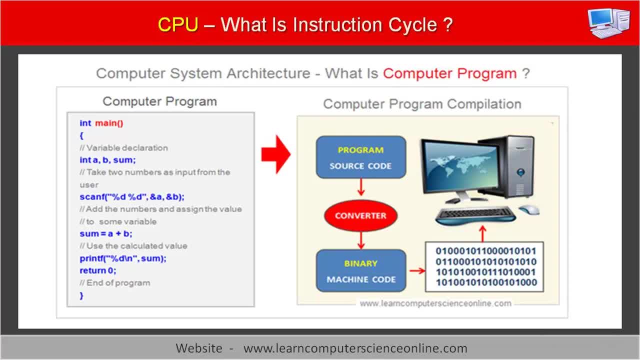 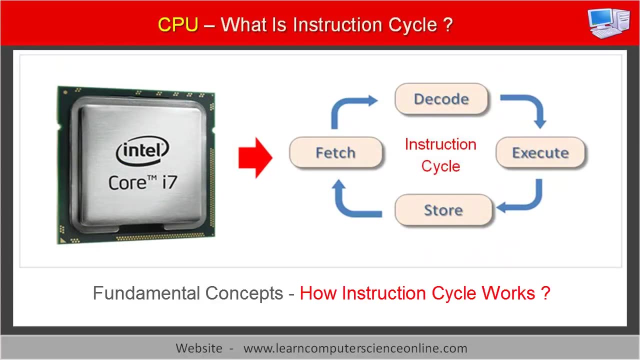 We will also discuss some important fundamental concepts, such as what are program instructions and how computer's microprocessor executes the program instructions. So let us first start with understanding some basic, fundamental, important concepts necessary to understand how instruction cycle works. 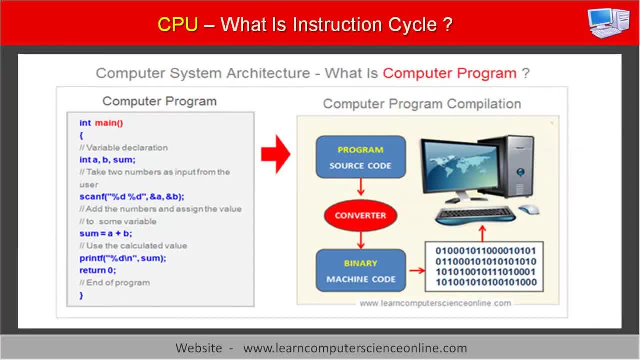 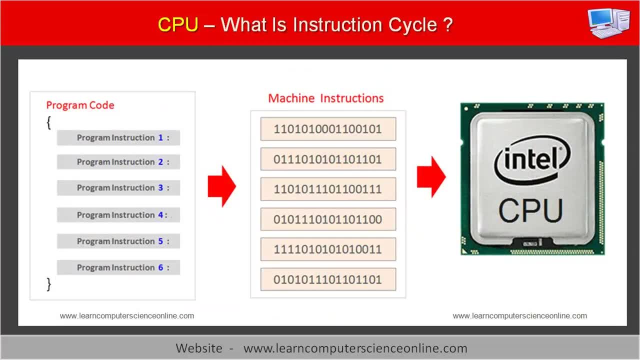 Let us first start by understanding what is a program instruction? The computer programs are an essential component of every computer system. The computer system needs a set of instructions which directs the computer to perform the desired operations. 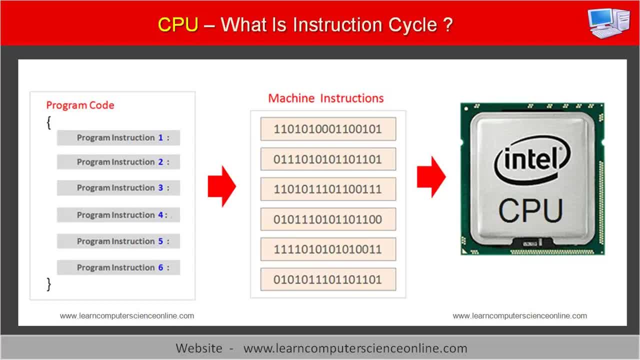 The computer programs writtenby using any high level programming language, such as C++, Java or Python. However, the computer understands only binary code, That is, a language of either 0 or 1. And therefore every high-level program needs to be first converted into a. 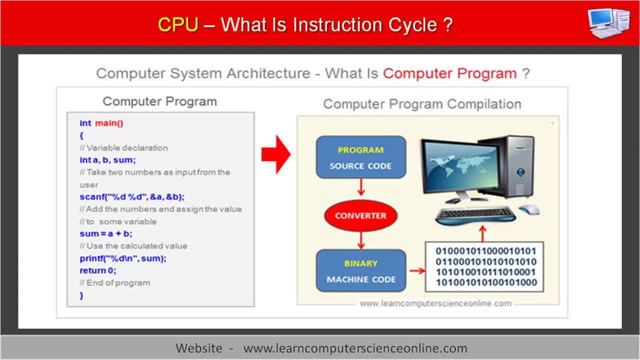 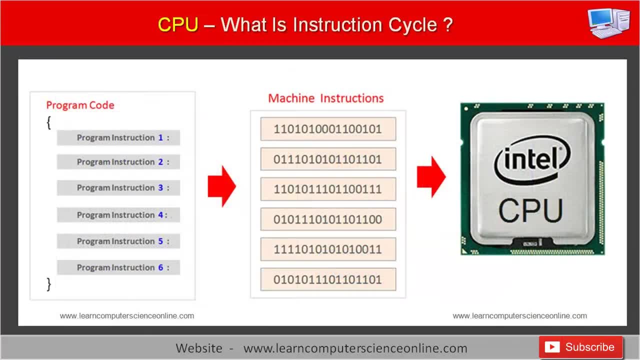 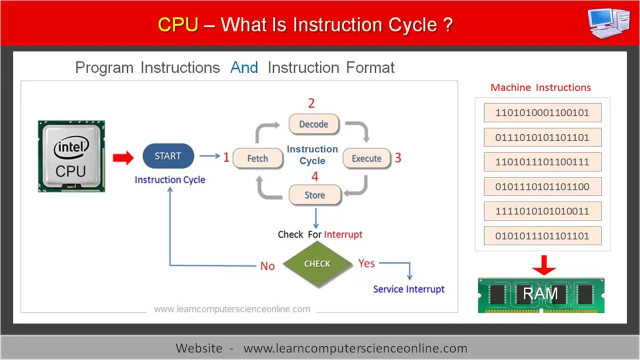 machine-readable instructions in binary that the processor can directly execute. The program instructions are an important part of the instruction cycle And therefore let us understand what are program instructions and what is instruction format. The computer program consists of group machine instructions stored into the main memory. Each machine instruction 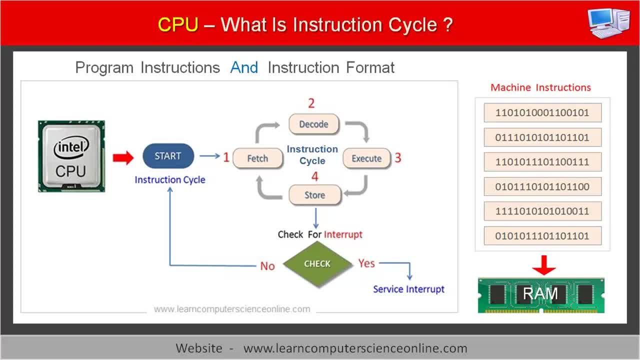 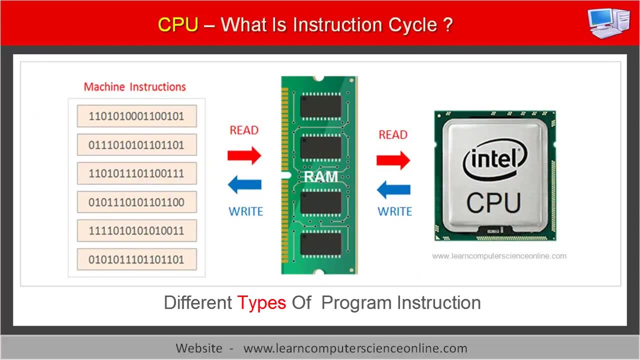 performs a specific task. The machine code instructions- a binary, a low-level set of program instructions- are the main instructions stored into the main memory. Each machine instructions are a custom-made instruction that can be directly executed by the computer system. The computer program makes use of different types of program instructions. 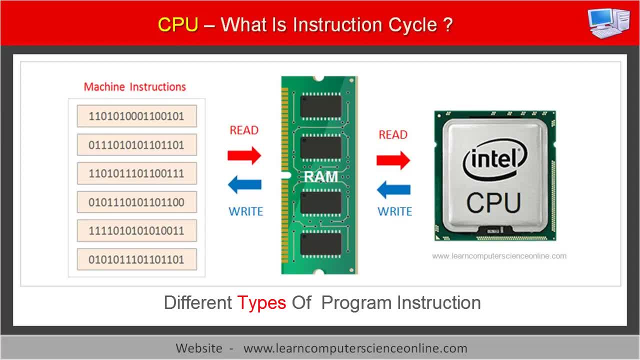 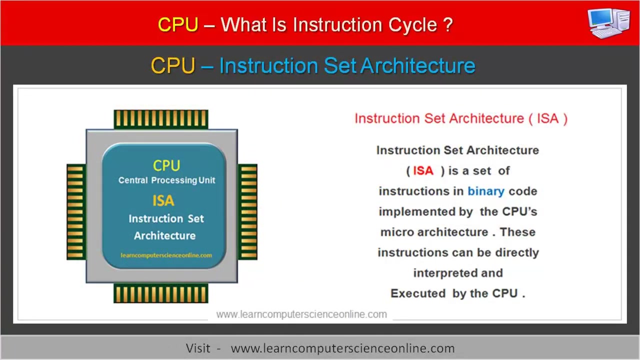 as per the program logic and algorithm. For example, the program instruction can either perform a memory-read, memory-write operation, input and output operations or arithmetic calculations, and some instructions Direct the CPU for performing logical operations such as decision-making operation. The CPU decodes the instruction as per the operation code specified in the instruction format. 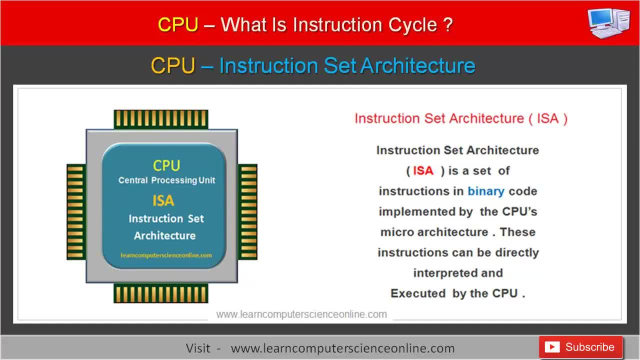 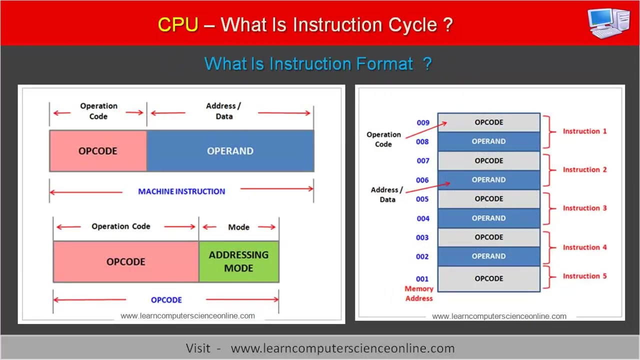 The processor executes the operation as per its internal set architecture ISA. The ISA is a set of binary commands that are supported by the processor. Each processor implements a set of binary commands called its internal set architecture ISA. The instruction format is another factor that plays an important role during the instruction cycle. 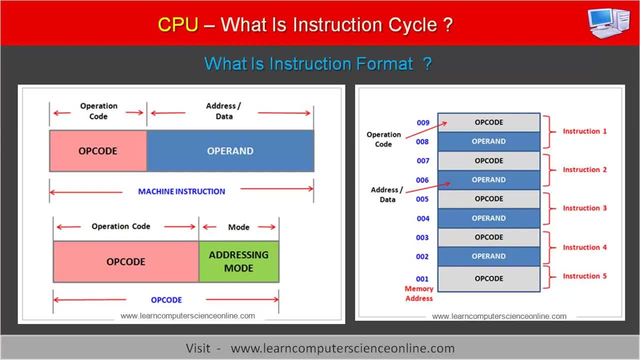 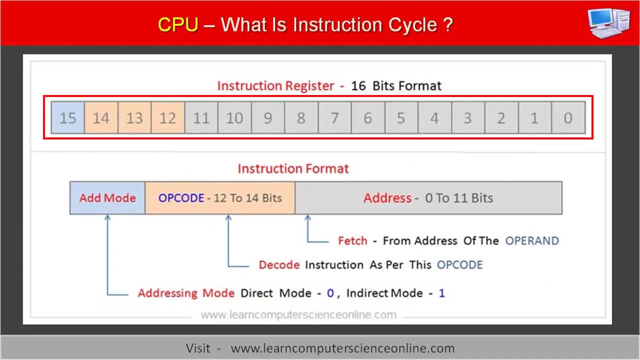 The instruction format directs the CPU during the instruction decode operation. In this example, the instruction format refers to the 16-bit instruction format. The 16-bit instruction format has three parts, or rather group of bits. Each part of the instruction format provides specific information to the CPU while decoding the instruction. 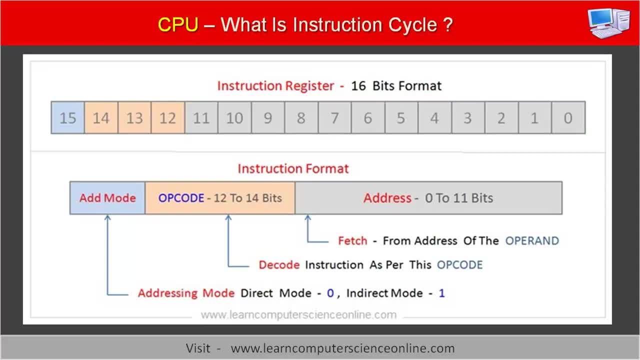 The first group of 12 bits, starting from 0-bit to 11-bit, indicates the address of the op-rand. The second group of 3 bits, starting from 12-bit to 11-bit, indicates the address of the op-rand. 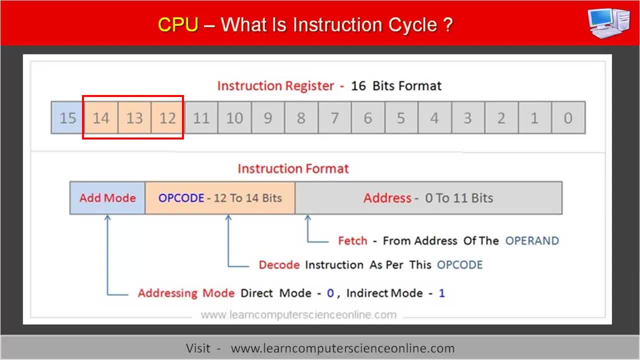 The third group of 3 bits, starting from 0-bit to 14-bit, indicates the operation code called as op-code, If the op-code defines the operation to be performed by the CPU. And the last bit, that is, 15-bit, indicates the addressing mode. 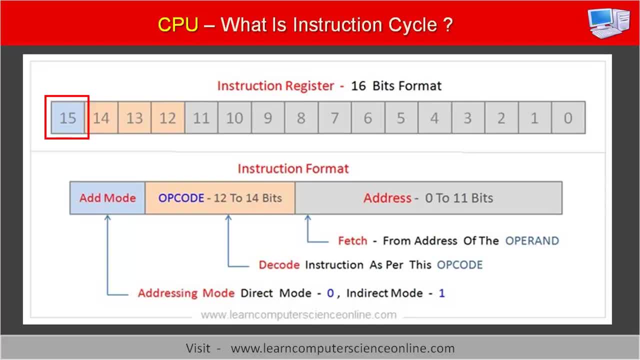 The addressing mode directs the CPU to either directly or indirectly fetch the value of the op-rand. The addressing mode bit 0 indicates the value of the op-rand. The addressing mode bit 0 indicates the value of the op-rand. The addressing mode bit 1 indicates the direct addressing mode. 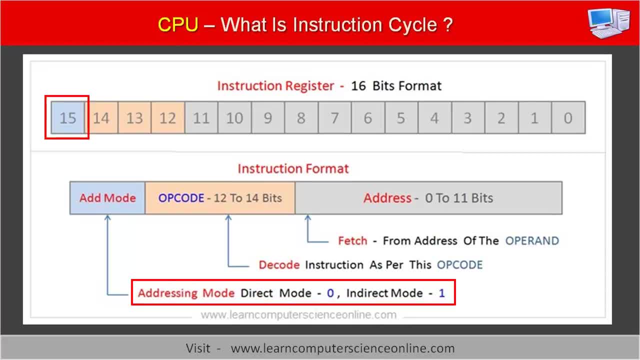 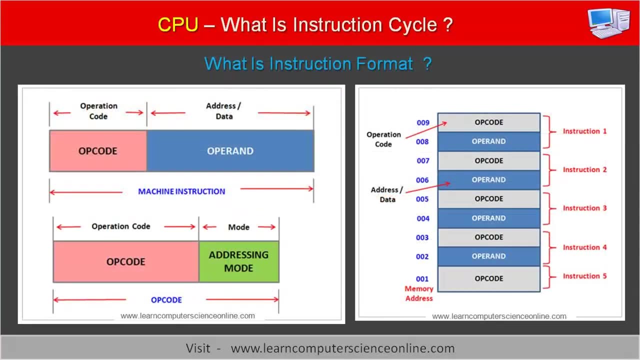 And the addressing mode. bit 1 indicates the indirect addressing mode. For indirect addressing mode, the CPU needs to first fetch the effective address and then fetch the value of op-rand from the effective address. Alright, so far, have learned what is instruction. 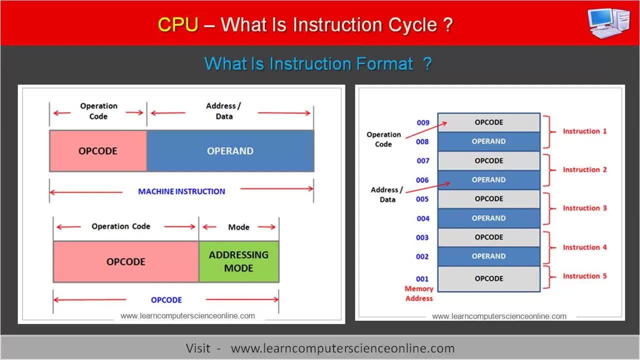 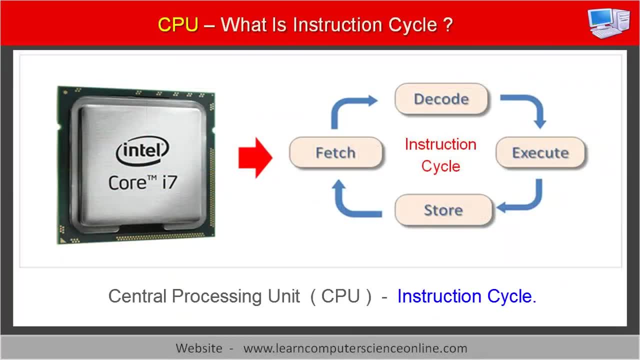 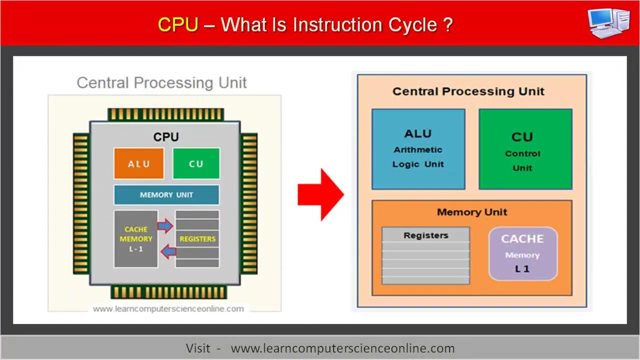 and how these instructions are decoded by the CPU with the help of instruction format. Let us now discuss what is instruction cycle. The instruction cycle is the basic operation of the CPU. It is the CPU that initiates and executes the program instructions, And therefore we need to study different components of the CPU that executes the instruction cycle. 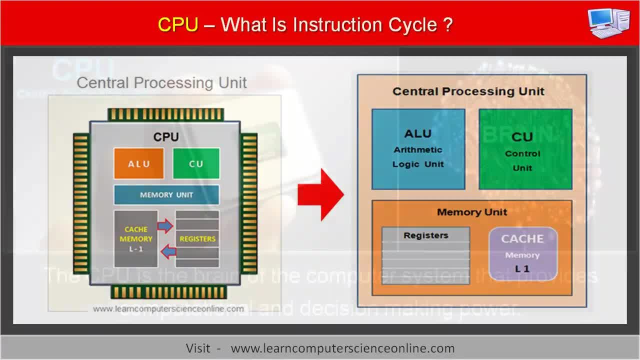 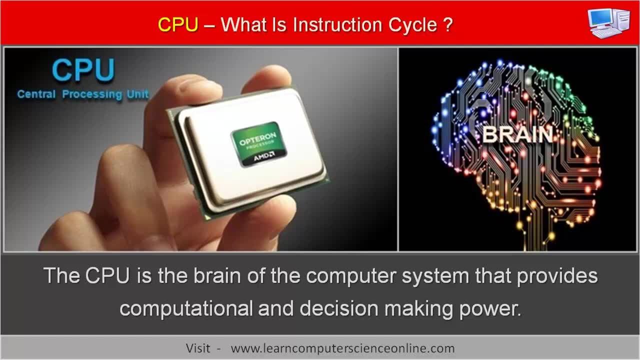 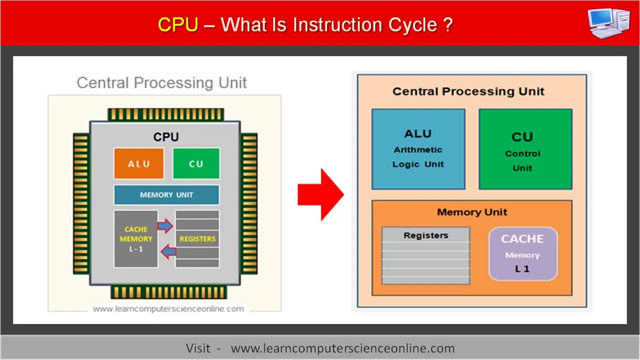 The CPU stands for Central Processing Unit. The CPU is the brain of the computer system, that provides the processing power to the computer system. It is the CPU that controls all the operations performed by the computer system, including the activities necessary to execute the program instructions. 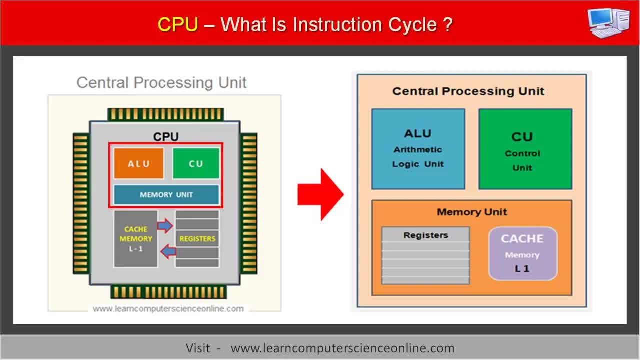 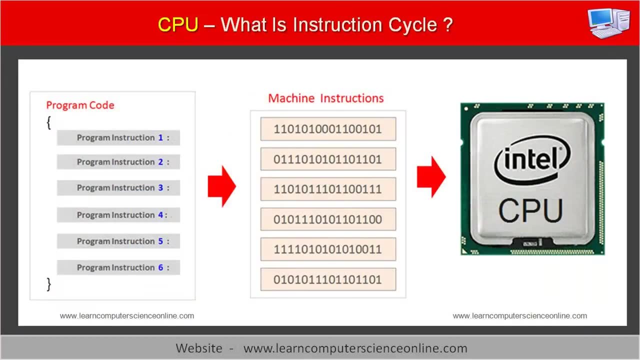 The CPU internally consists of three important units. These three units are called CPUs. These three CPU internal components are: first, memory unit, second, control unit and third, arithmetic and logic unit. So far we have discussed what are program instructions and the CPU. 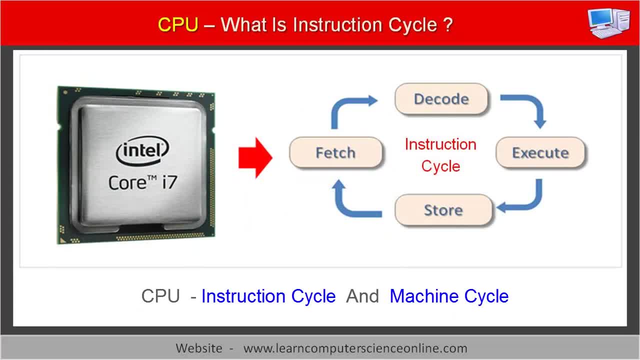 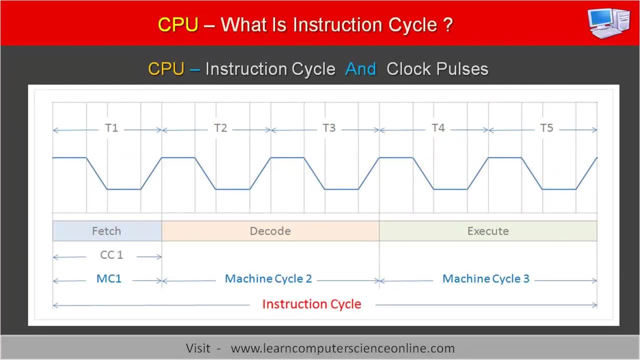 Let us now discuss in detail what is machine cycle and the instruction cycle. Let us first start with understanding what is instruction cycle. The instruction cycle is the time required by the CPU to execute one single instruction. The instruction cycle is also commonly referred to as machine cycle. 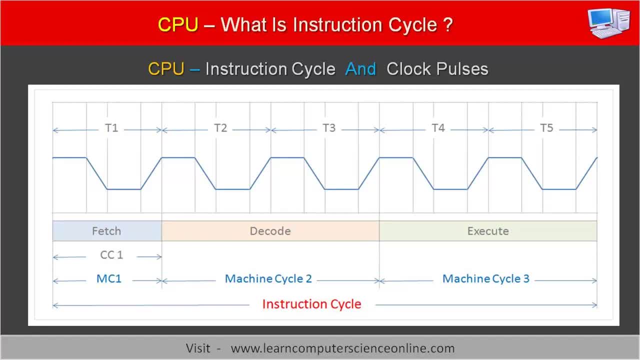 but there is a difference between these two CPU operations. The instruction cycle consists of three steps. The first phase of the instruction cycle is to fetch the instruction. The second phase is to decode the instruction. The third phase is to execute the instruction, And therefore the instruction cycle is often referred as fetch, decode, execute cycle. 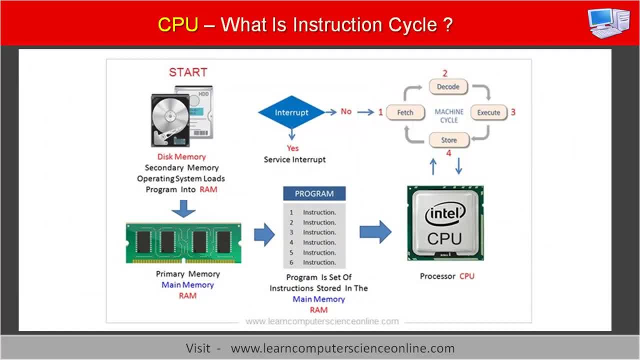 Let us now understand the instruction cycle execution step by step. The computer starts the program execution when the operating system loads the executable copy of program into the main memory RAM. The executable copy of the program loaded into the memory consists of set of machine instructions that can be directly executed by the CPU. 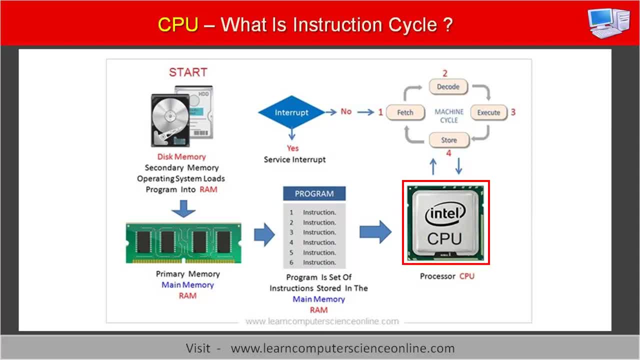 The CPU starts the execution of the instruction cycle by fetching the machine instructions from the memory one by one. The entire instruction cycle execution by the processor can be split into three separate operations. These operations include the fetch operation, the decode operation and finally the execute operation. 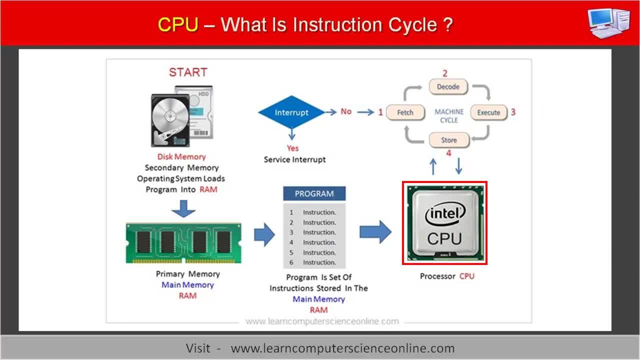 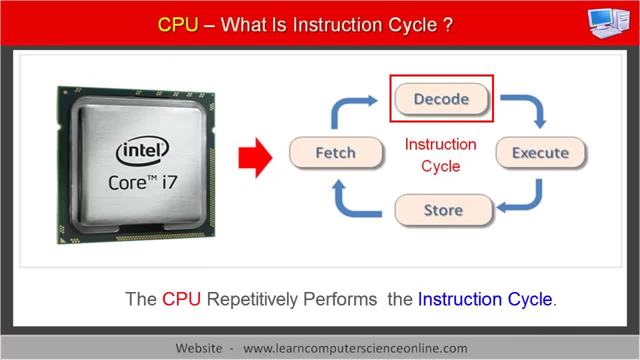 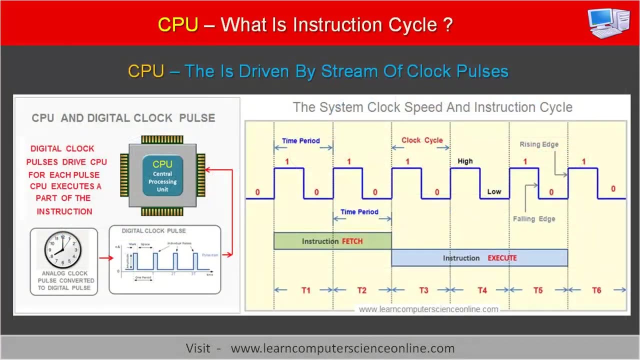 The CPU also stores the result into the memory. after the execute operation, The CPU repetitively perform the instruction cycle to execute the program instructions and also for other operations of the processor. The processing speed of the processor depends upon the off frequency of its internal clock. 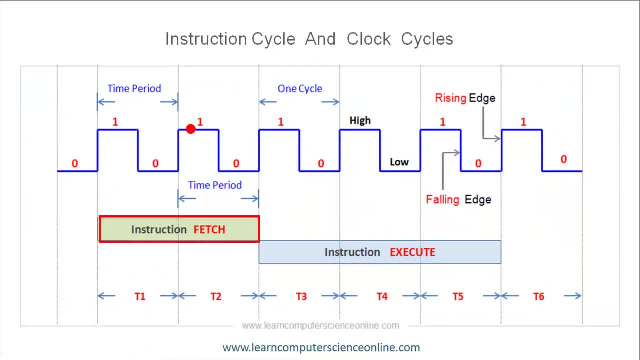 The CPU is driven by the steam of clock pulses generated by the quartz clock built into the processor chip. For each clock pulse, the CPU executes a part of the instruction cycle. The clock pulse time uniformly divides the processing time required to execute the instruction cycle by the processor. 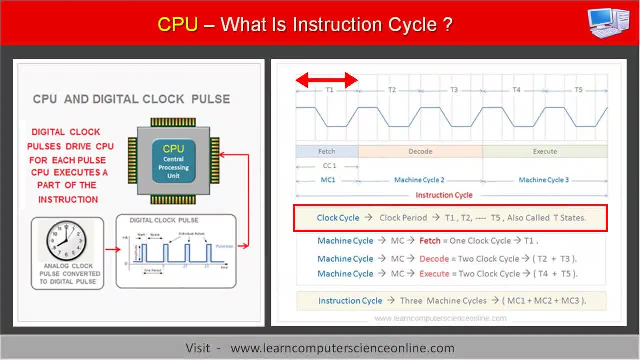 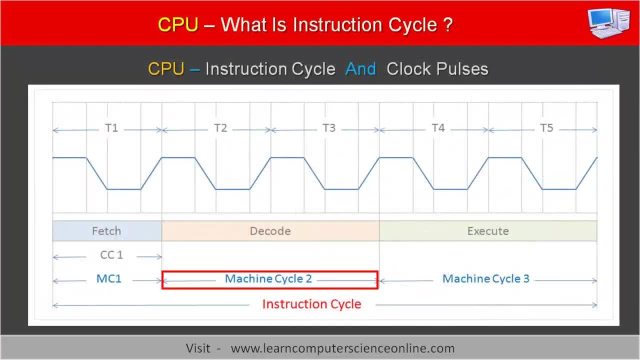 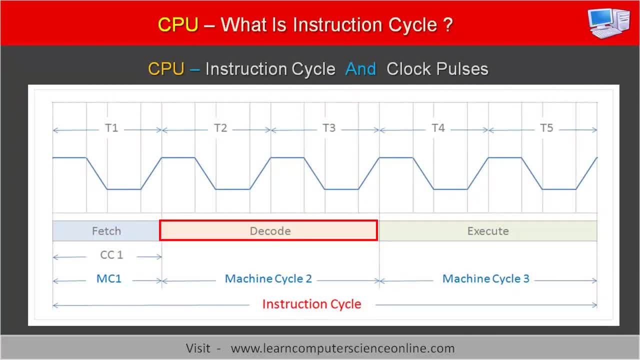 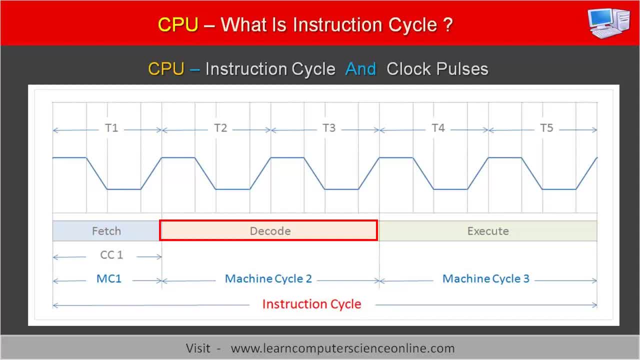 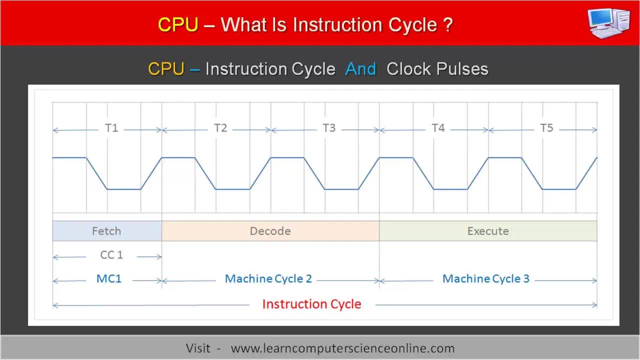 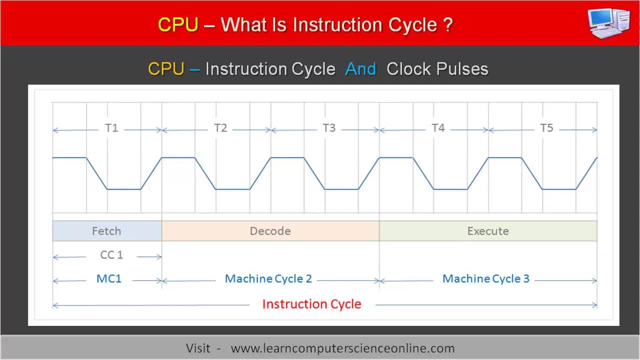 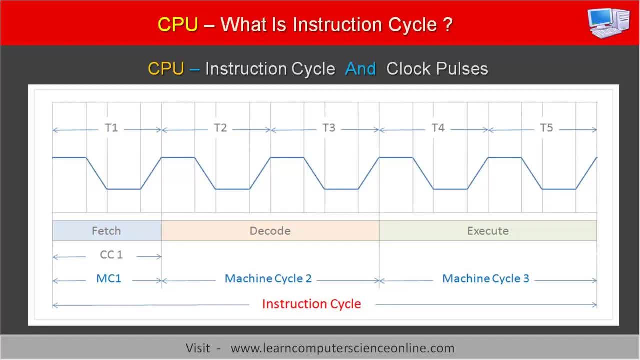 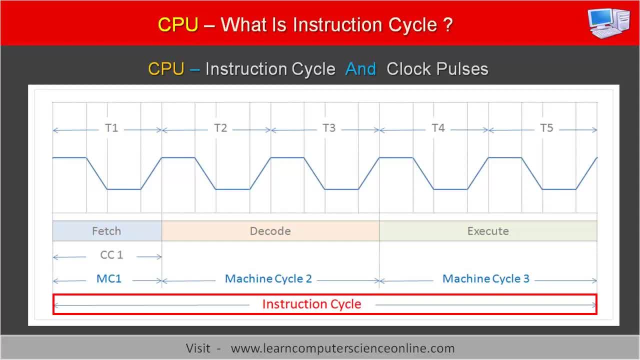 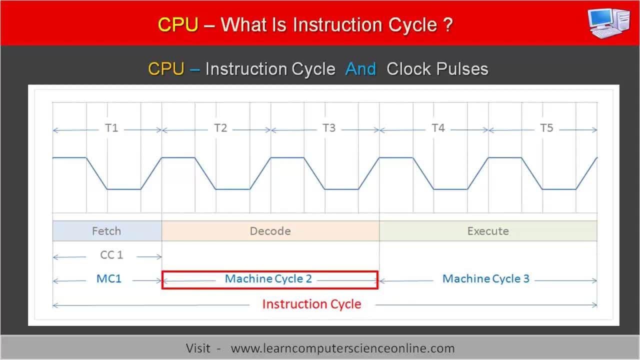 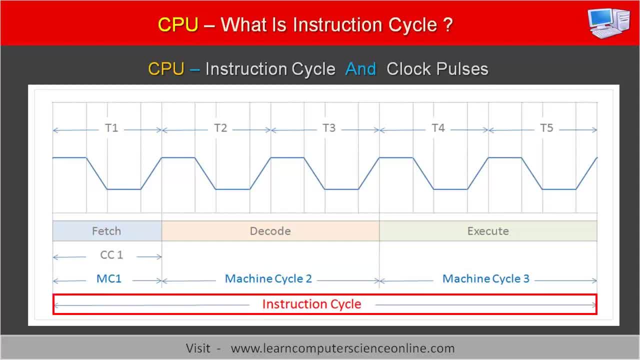 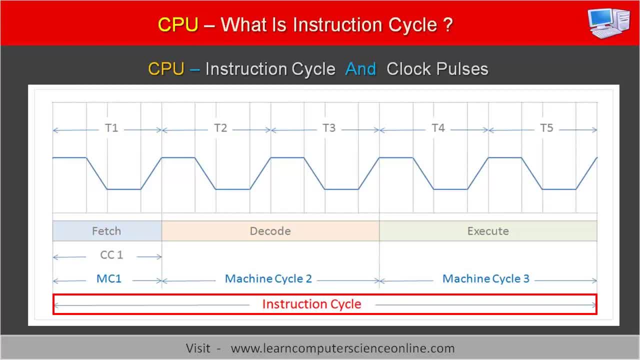 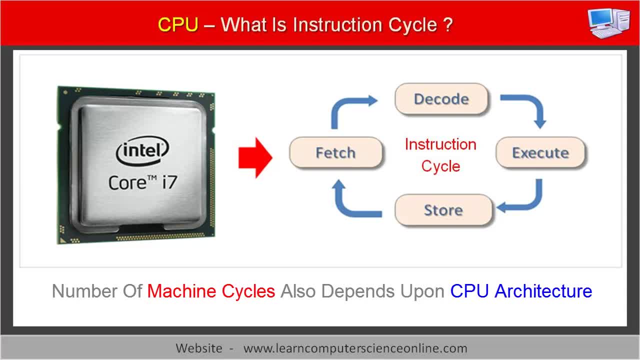 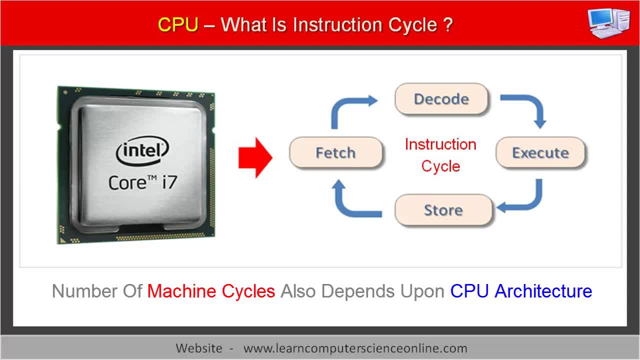 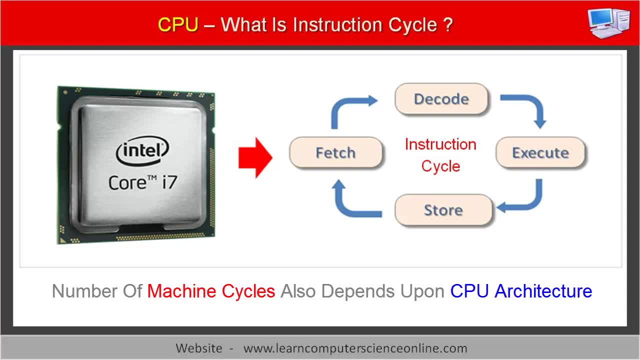 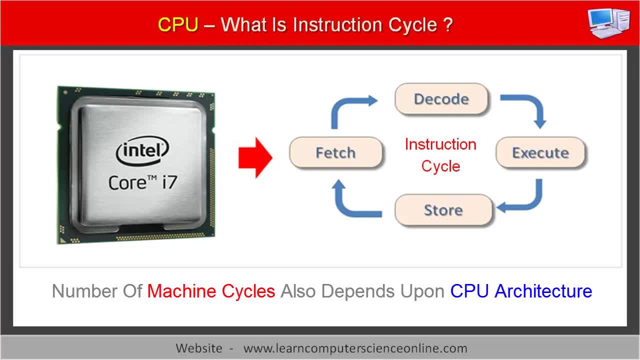 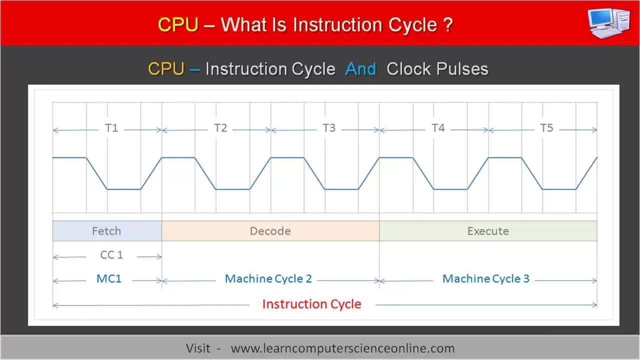 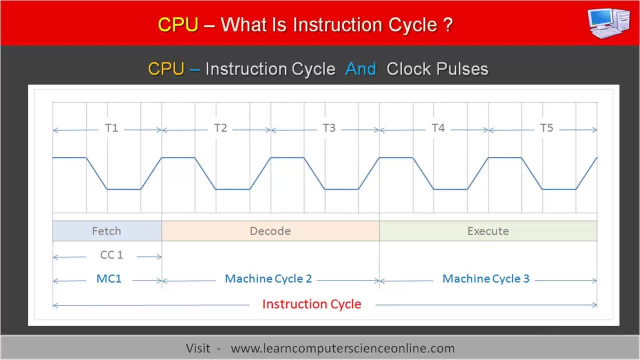 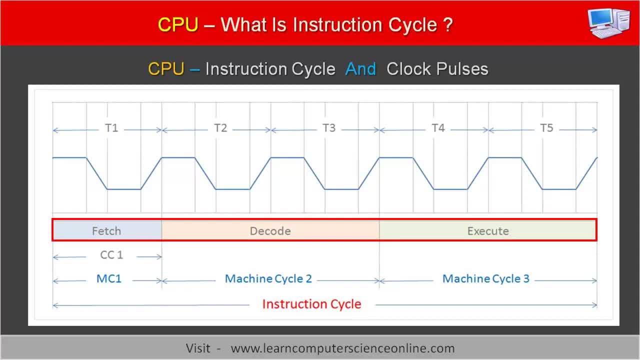 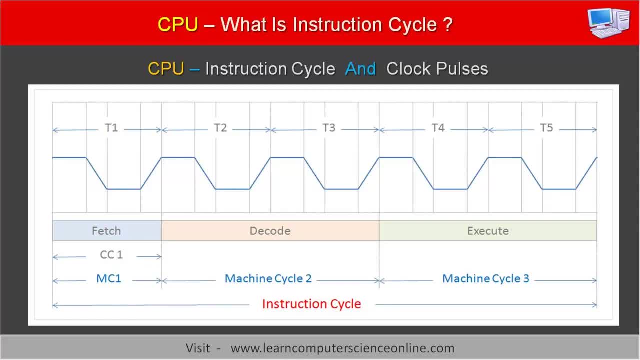 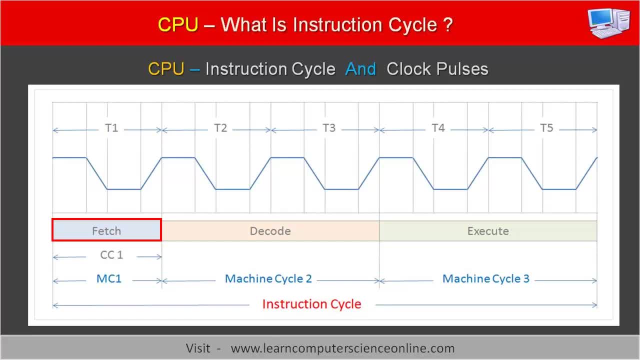 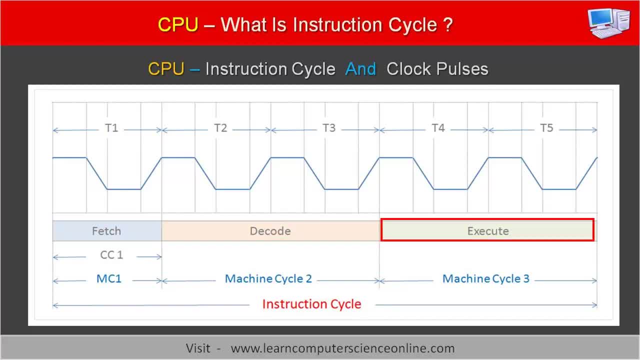 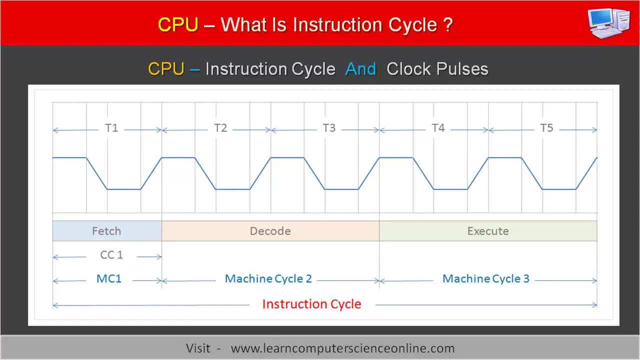 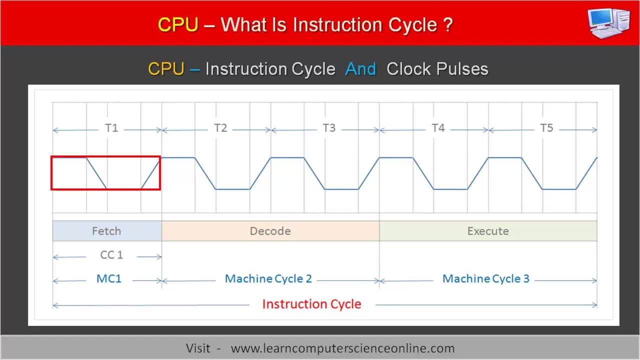 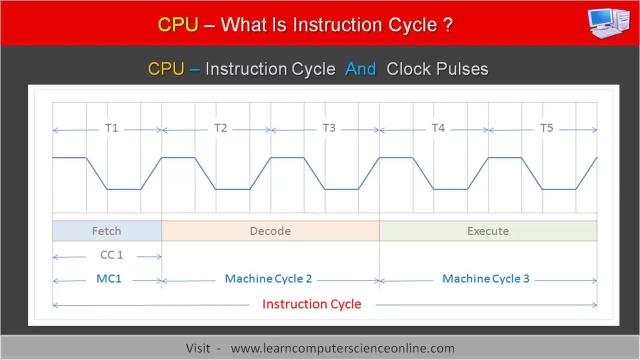 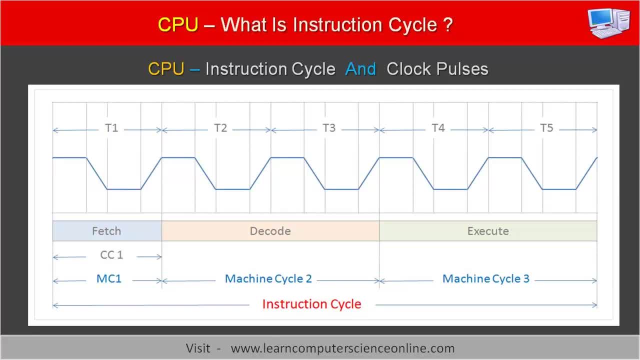 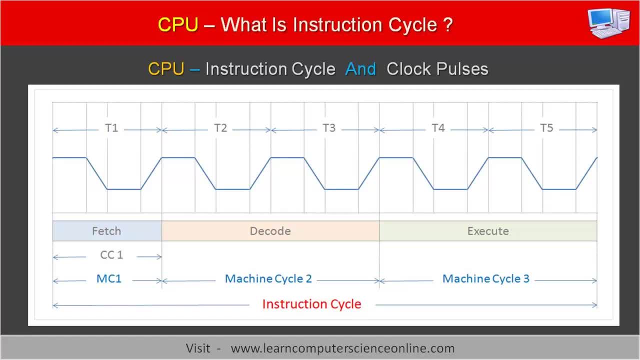 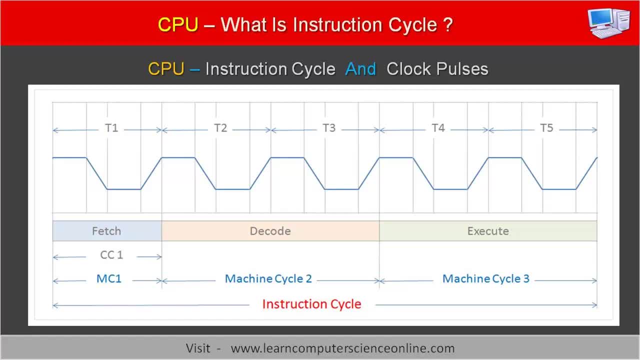 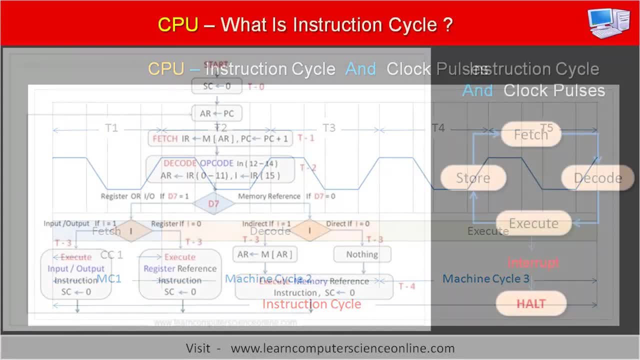 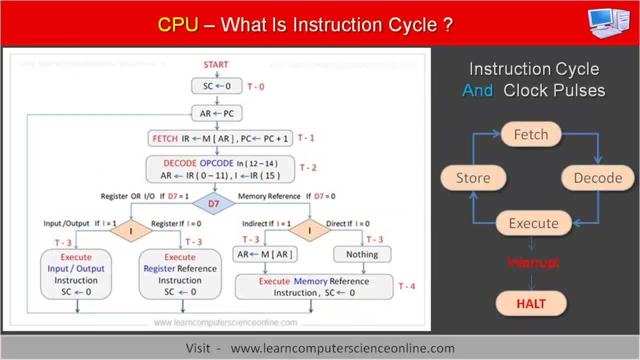 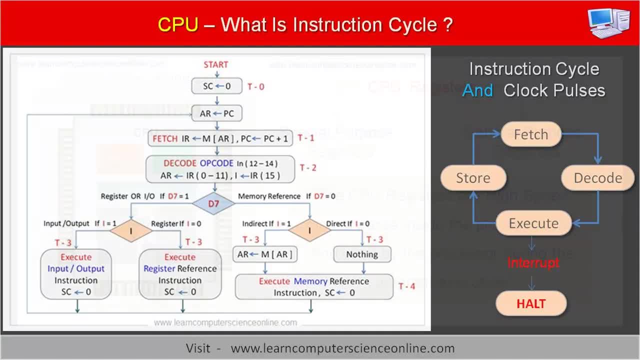 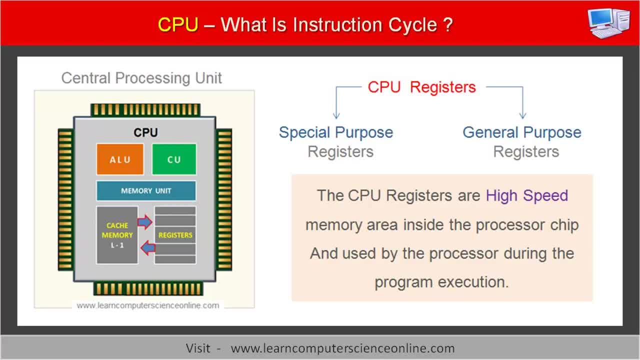 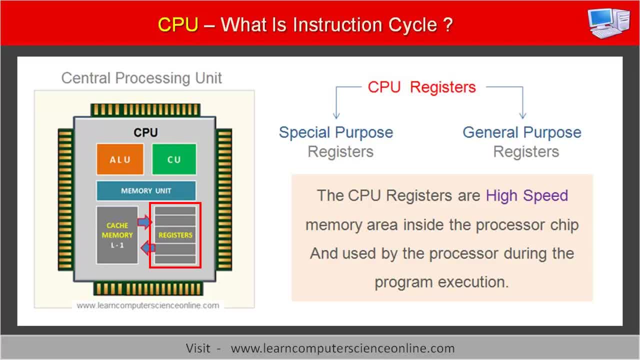 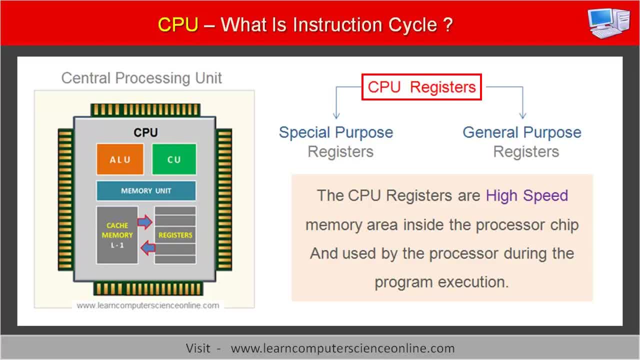 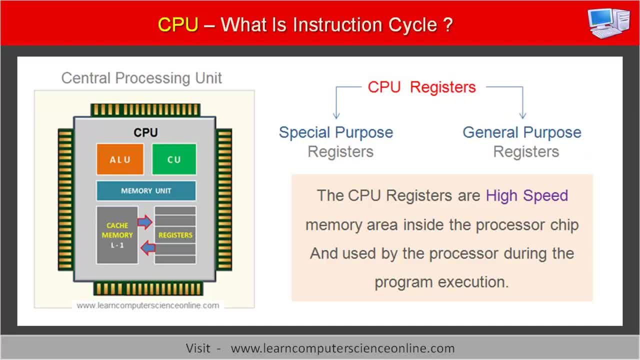 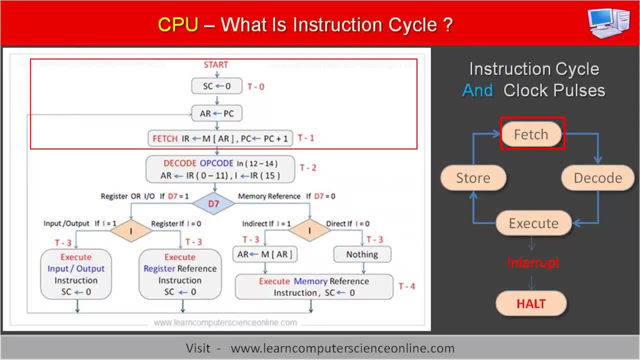 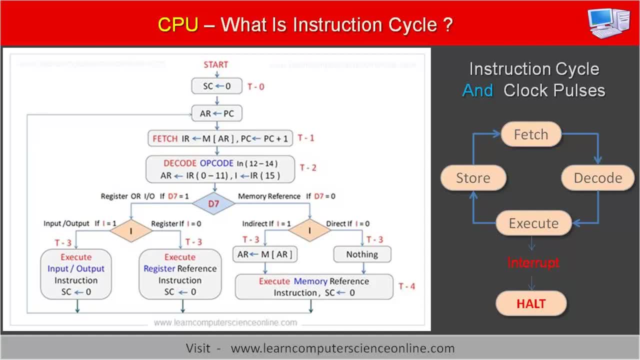 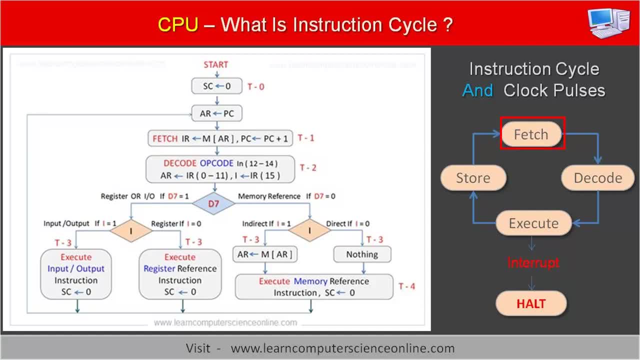 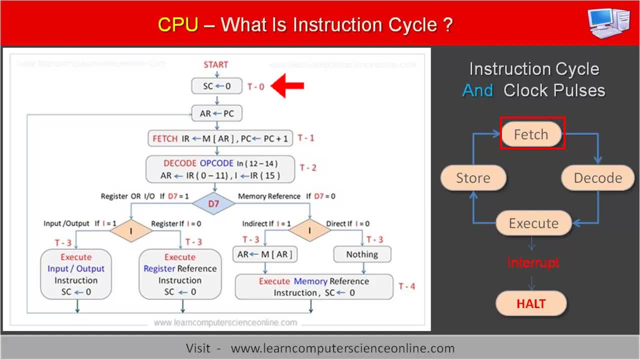 The term machine cycle refers to the execution of part of the instruction cycle operation. The term machine cycle refers to the execution of part of the instruction cycle operation to 0 at clock cycle T0.. The program counter register PC always contains the address of the next instruction in the pipeline In the first clock cycle at. 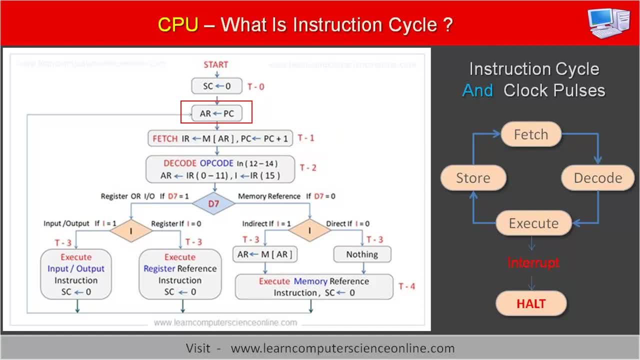 clock pulse T0,, the content of the program counter register PC will be assigned to the address register RR. In the next clock cycle, that is, at clock cycle T1, the instruction is fetched from the main memory RAM and brought to the instruction register IR and at the same time the program counter register. 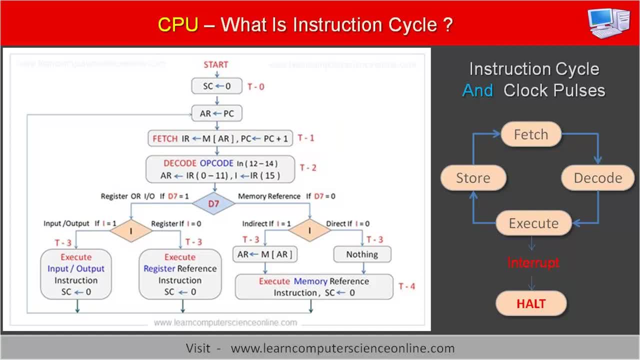 PC is incremented by 1.. The program counter PC now points to the next instruction to be fetched from the memory. At this stage the fetch operation of the instruction cycle ends And the decode operation starts. The second phase of the instruction cycle is. 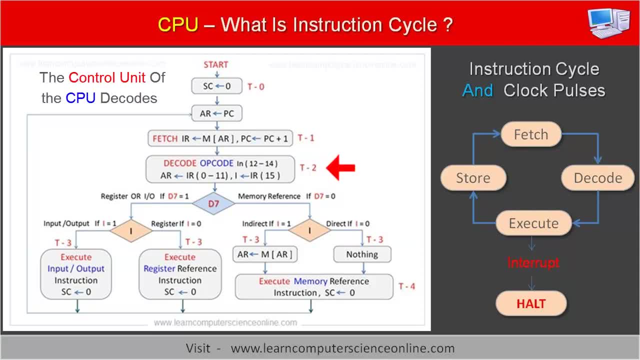 called the decode operation, The control unit of the CPU decodes the program instruction placed into the instruction register IR. during the fetch operation, The CPU decodes the instruction as per the instruction format. The instruction format defines the operation to be performed by the CPU. 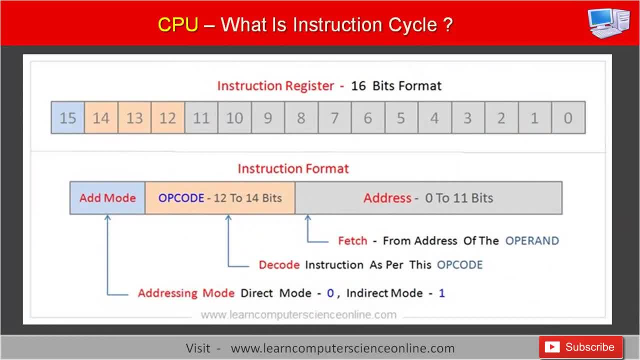 The instruction format directs the CPU in terms of, first, the addressing mode, second, the memory address of the operand and, third, the operation that needs to be performed by the CPU. The instruction is decoded by the control unit of the CPU as per the operation code specified by the three bits, that is, bit number. 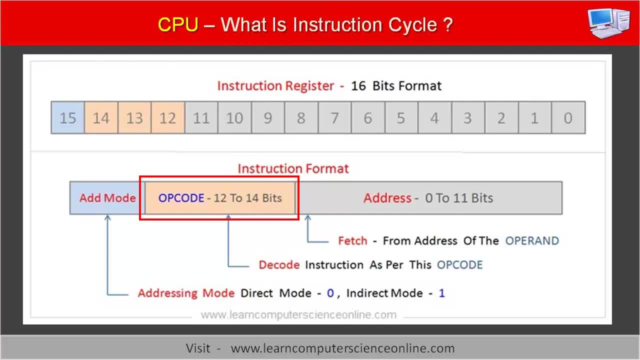 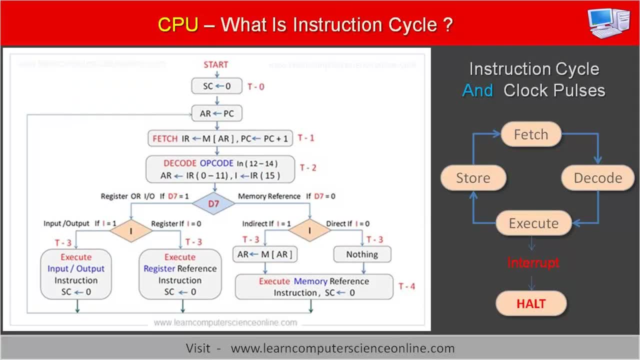 12,, 13, and 14, of the instruction format. Now the control unit has to first decide the type of the instruction. There are three types of instructions. The first type is memory reference instruction. the second type is register reference instruction. and the third type is input and output instruction. 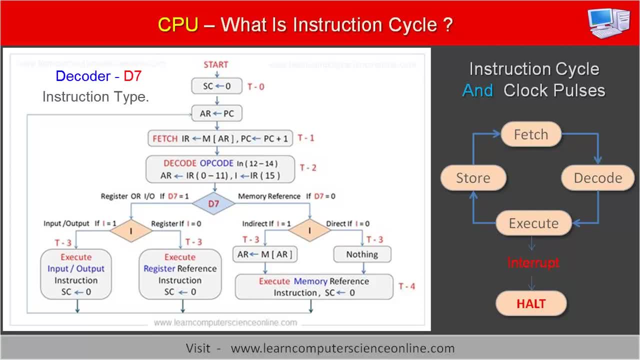 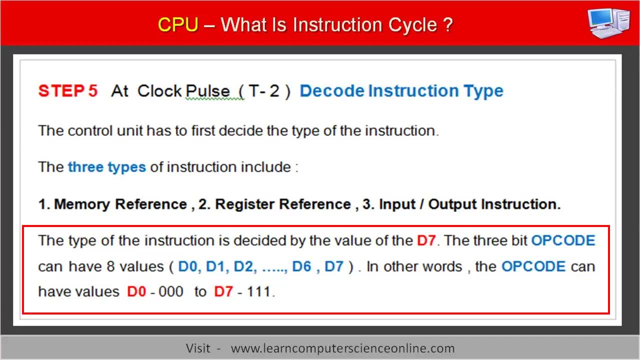 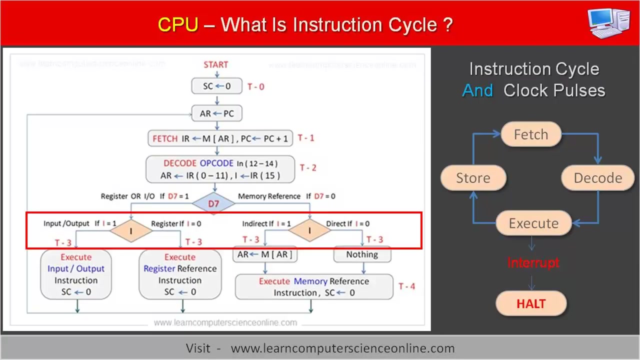 The type of the instruction is decided by the decoder as per the value of D7.. The three-bit opcode can have eight possible values, starting from D0,, D1,, D2, till D7. In other words, the opcode can have values from 000 to 111.. The next step is to decode the addressing. 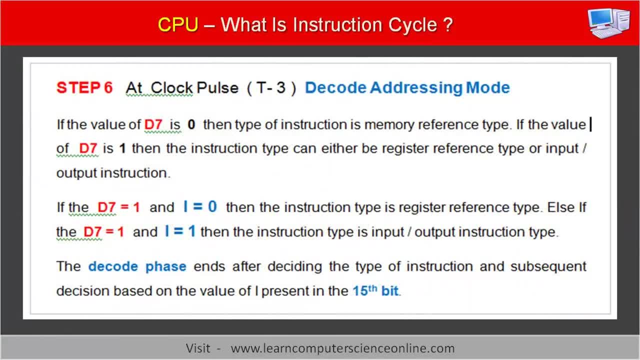 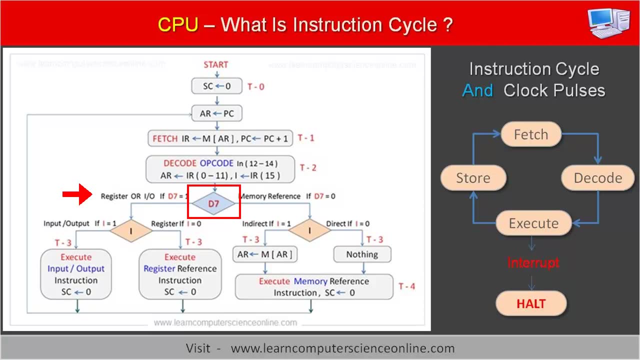 mode at clock pulse T3.. If the value of D7 is equal to 0,, then the type of instruction is considered as memory reference type. However, if the value of D7 is equal to 1,, then the instruction type can either be register: 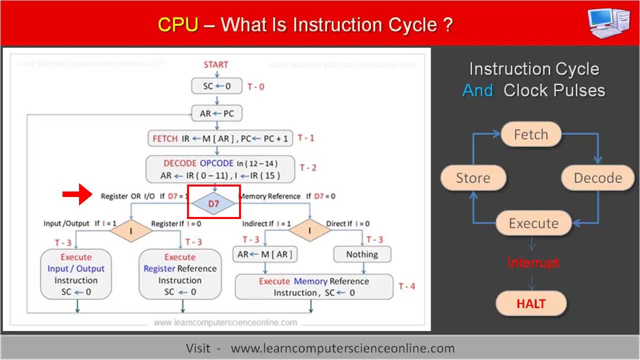 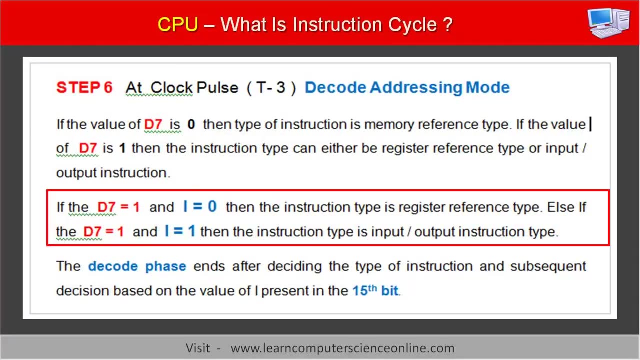 reference type or input output instruction type. At this stage, the CPU refers to the value of the 15th bit of the instruction format. If the value of D7 is equal to 1 and the value i is equal to 0,, then the instruction type is considered as memory reference type. 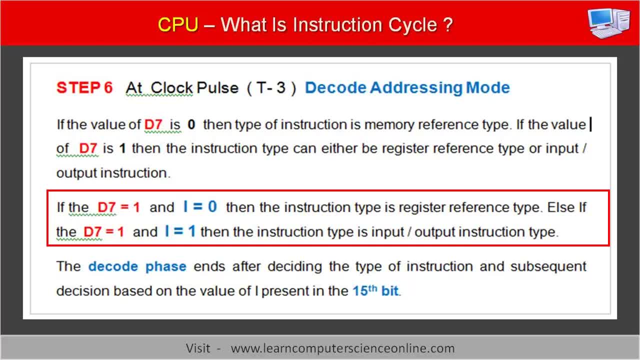 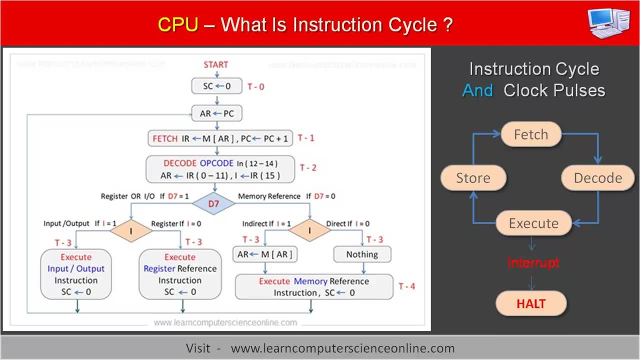 The third type is the input and output instruction type. But if the value of D7 is equal to 1 and the value of i is equal to 1, then the instruction type is considered as input output instruction type. The decode phase of the instruction cycle ends after deciding the type of instruction and 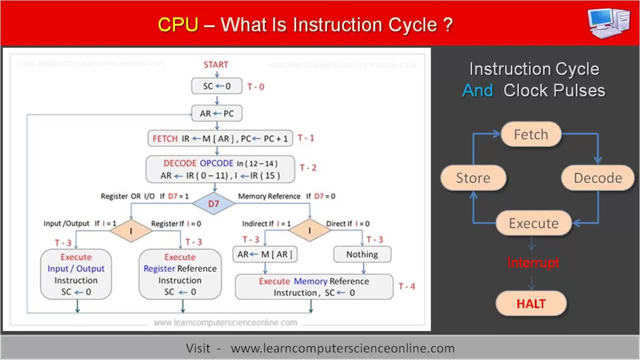 subsequent decision based on the value of the. i present in the 15th bit For the memory In memory reference instructions. the decode operation decides the addressing mode of the instruction. The addressing mode for memory reference type depends upon the value of. i present in the 15th bit of the instruction format. 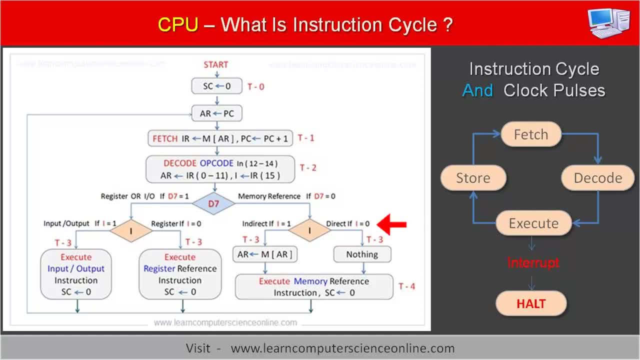 If the value i is equal to 0, then the addressing mode is considered as direct. The addressing mode is considered as indirect if the value of i is equal to 1.. At this stage the decode phase of the instruction cycle ends and now the execution phase starts. 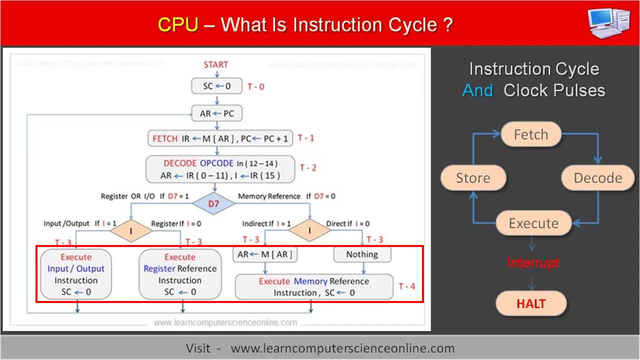 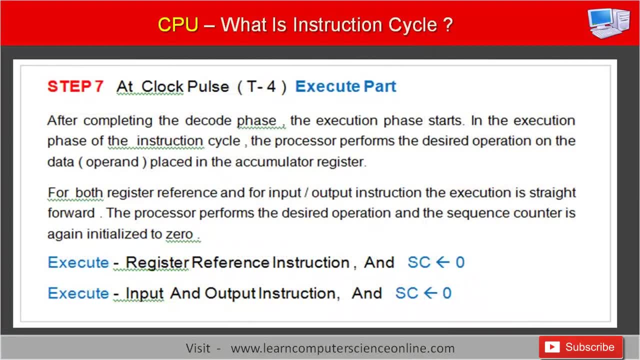 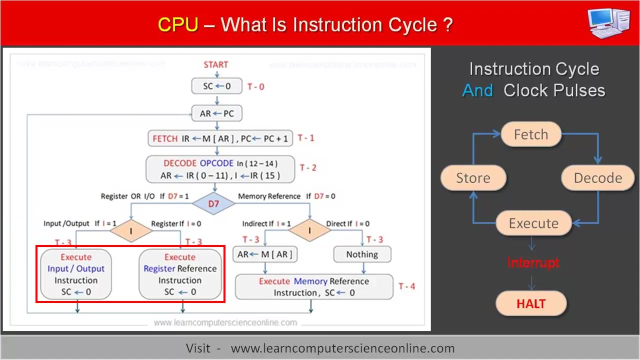 After completing the decode phase, the execution phase of the instruction cycle starts. In the execution phase of the instruction cycle, the processor performs the desired operation on the fetched data For both register reference and also for input-output instruction. the execution operation by the CPU is straightforward operation. 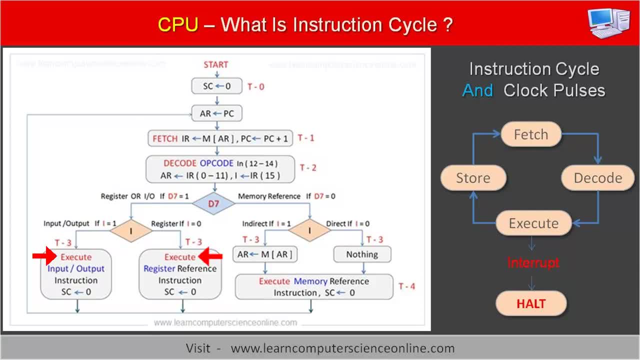 And in such cases the processor performs the desired operation and the sequence counter is again initialized to 0.. For memory reference instruction, the 15th bit- addressing mode- of the instruction format, decides the direct or indirect execution. that depends upon the addressing mode. 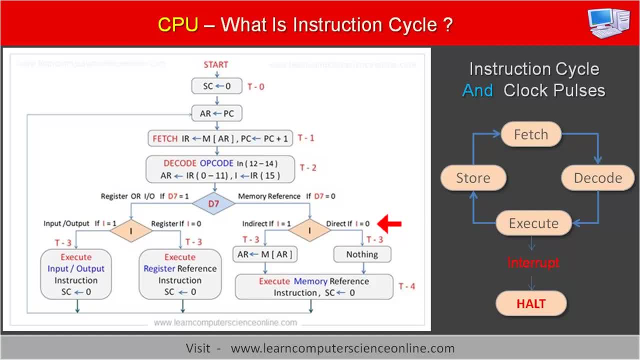 In case of direct referencing, the value of i is equal to 0, and the processor executes the desired operation on the data fetched from the address specified by the bits 0 to 11.. And the sequence counter is again initialized to 0.. 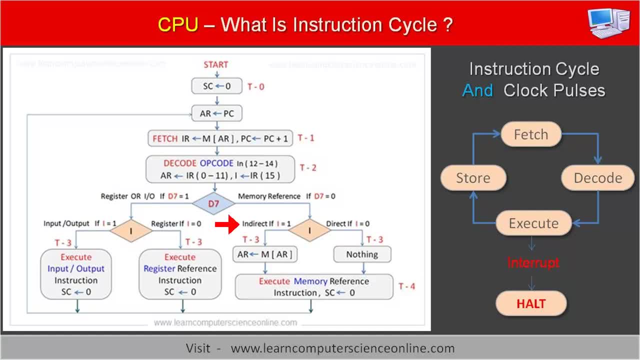 However, in case of indirect referencing, the value of i is equal to 1.. And the effective address of the operand is first located. The processor then executes the desired operation on the data fetched from the effective address as specified by the bits 0 to 11,. 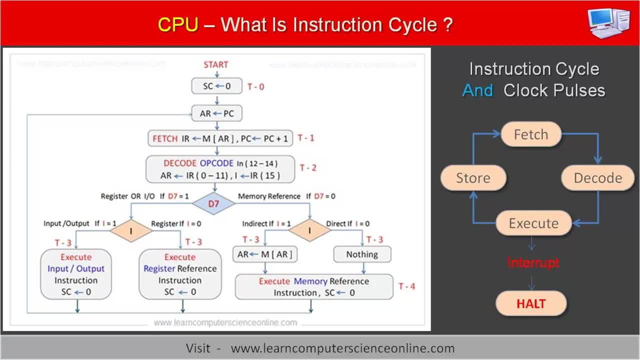 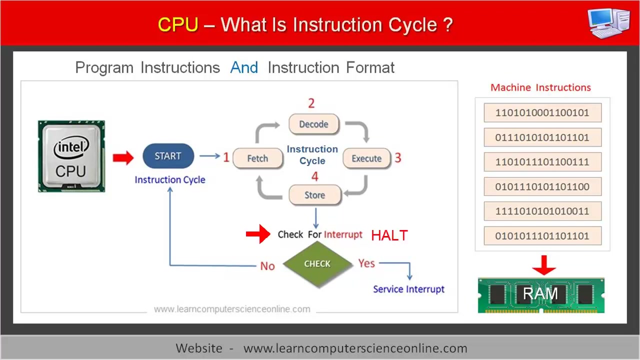 which points to the effective address, And the sequence counter is again initialized to 0.. After completing the execution phase of the instruction cycle, the control again goes back to the fetch phase, where the instruction cycle again starts. However, the instruction cycle can go to halt phase after the completion of the execution phase if it encounters.